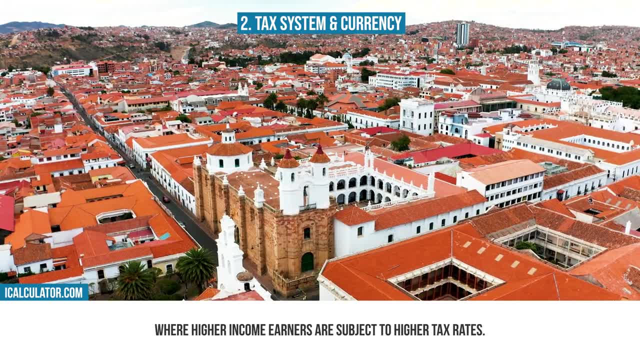 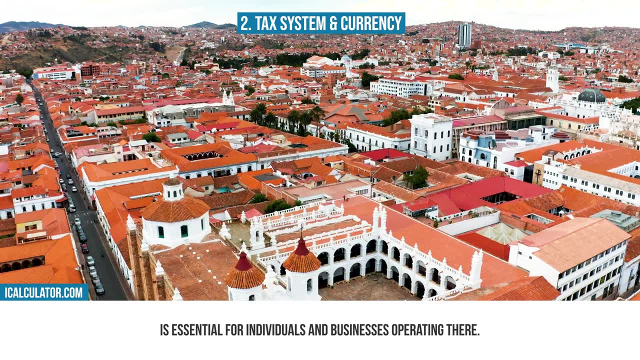 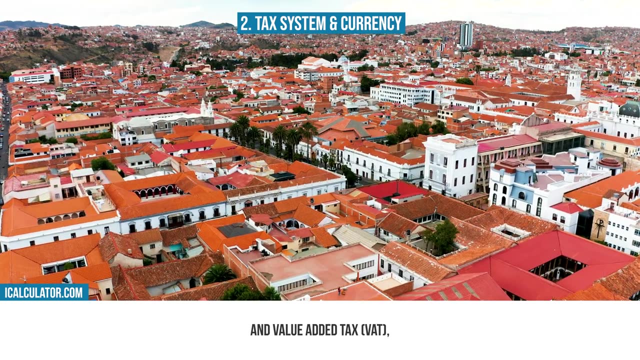 a progressive income tax structure where higher income earners are subject to higher tax rates. Understanding the tax year in Bolivia, with its specific deadlines and regulations, businesses operate there. The Bolivian tax regime includes personal income tax, corporate tax and value-added tax, aimed at supporting its economy and public services. 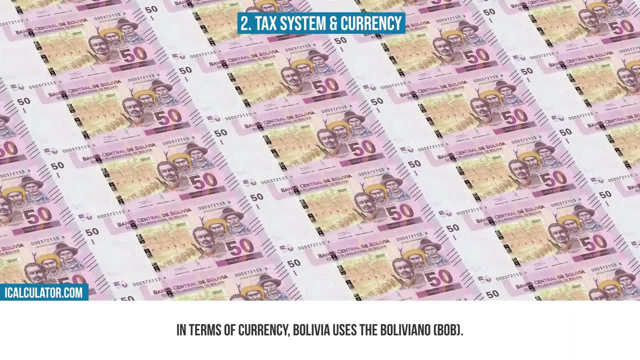 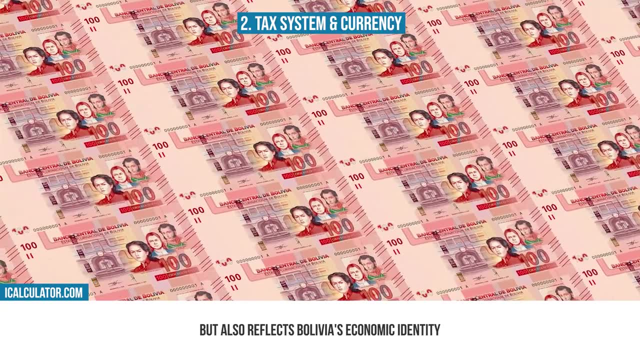 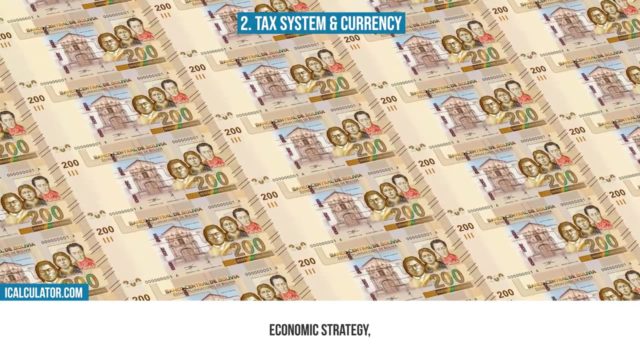 In terms of currency, Bolivia uses the Boliviano. The Boliviano not only facilitates everyday transactions, but also reflects Bolivia's economic identity and its efforts towards financial stability. The adoption of the Boliviano is a key element in Bolivia's economic strategy. 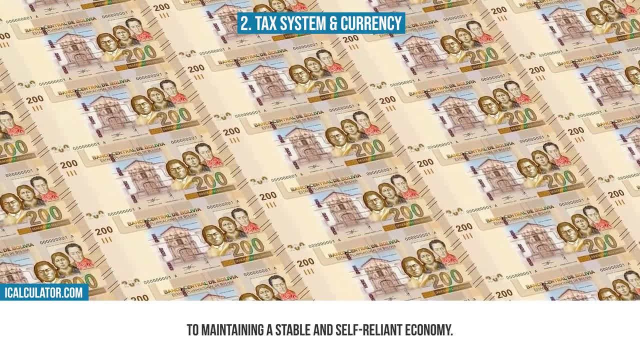 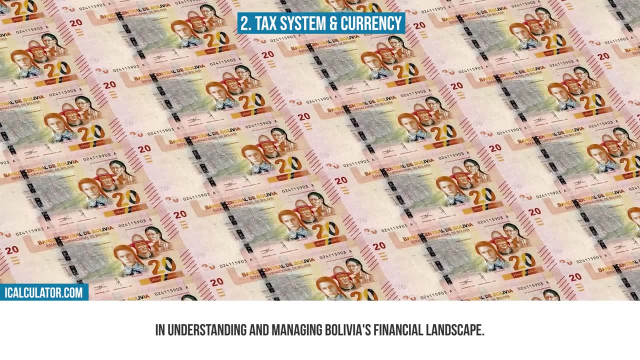 signifying its commitment to maintaining a stable and self-reliant economy. Next, let's look at how iCalculator tools can help you in understanding and managing Bolivia's financial landscape. iCalculator is home to a comprehensive suite of different tools to simplify and clarify. 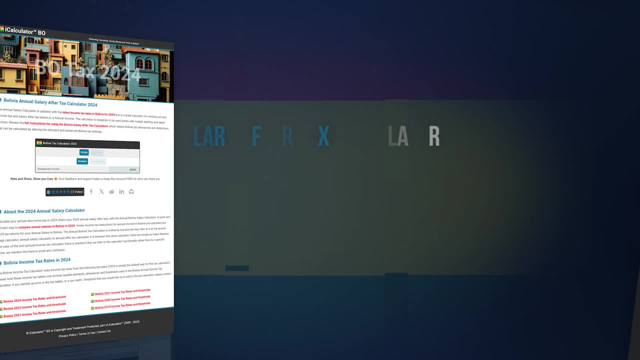 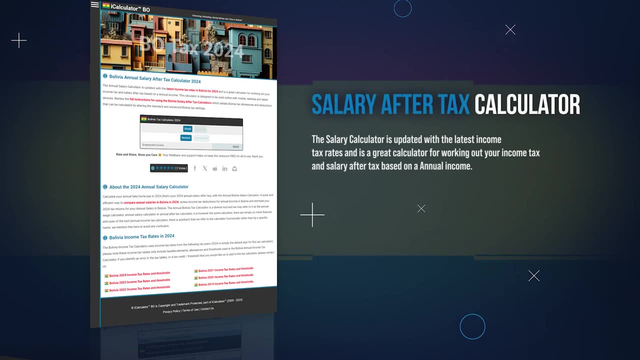 your financial planning and decision-making. You can start by understanding your take-home pay with our Salary After Tax Calculator, which offers a clear view of your net income after all tax deductions. Compare different salaries with our Salary After Tax Calculator, which offers a clear. 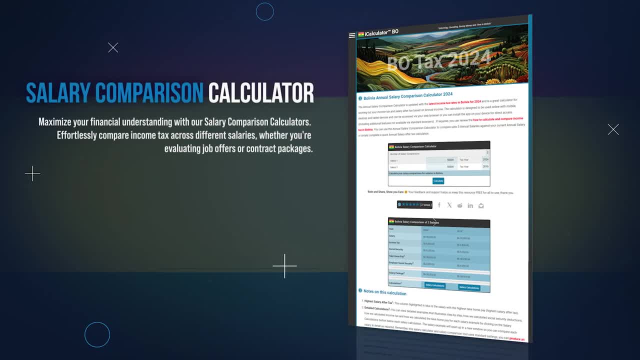 view of your net income after all tax deductions. Compare different salaries with our Salary After Tax Calculator, which offers a clear view of your net income after all tax deductions. Compare different salaries with our Salary After Tax Calculator, which offers a clear view of your net income after all tax deductions. Stay informed with our Sallary Comparison. 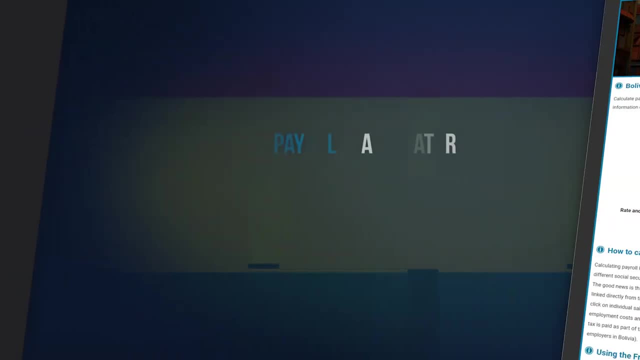 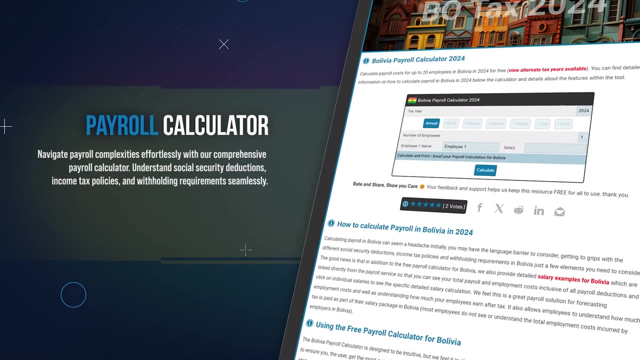 Calculator providing insights into where your earnings stand compared to previous years. Streamline your Payroll process using our Payroll Calculator, which is crafted to assist in calculating salaries, taxes and contributions for businesses. You can estimate the total cost of new hires using our Recruitment Cost Calculator, covering 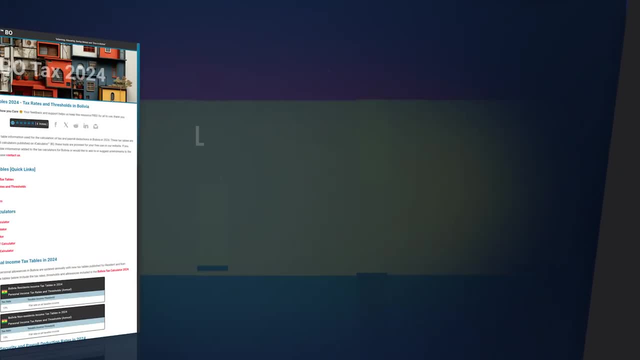 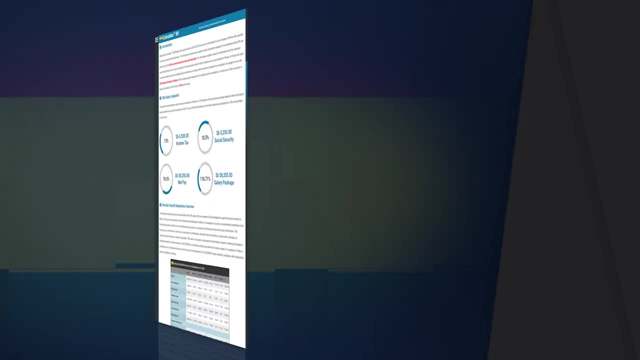 all aspects of the recruitment process. Stay informed with our tax tables offering a quick reference to the tax rates and thresholds from current and previous years. Explore a variety of salary scenarios with our salary examples offering detailed breakdowns of tax obligations for different wages. 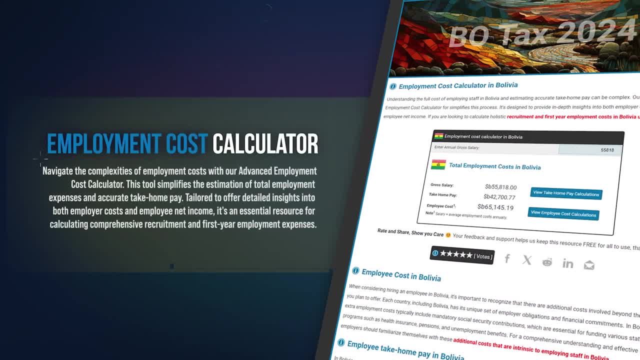 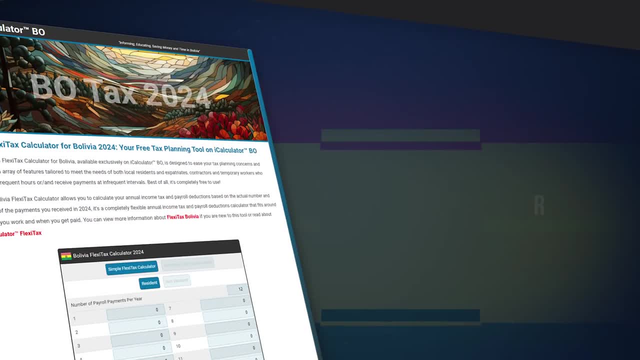 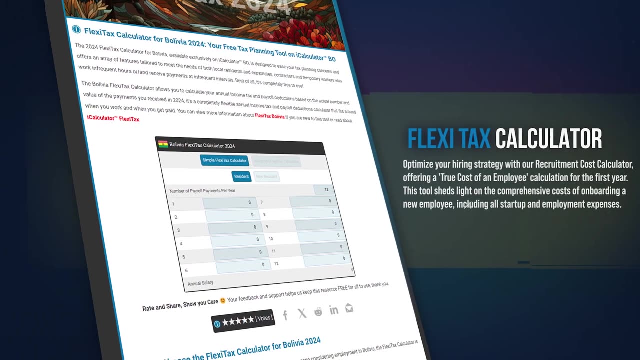 For employers, understand the full cost of employing staff with our Employment Cost Calculator, including salaries and additional benefits. And for those with irregular income, use our FlexiTax Calculator, a specialised tool for calculating salaries after tax for inconsistent income. Access all these tools easily with our free iCalculator app, available on all devices.